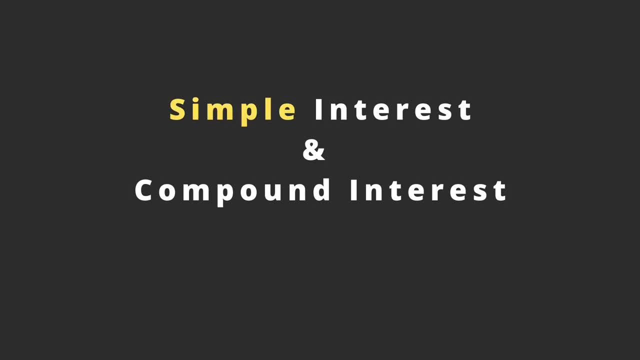 Hey guys, today we're going to go through different problems for simple and compound interest, which actually has a lot of real-world examples and applications. For example, if you put your money into a savings account at the bank, they will pay you what's called an interest for. 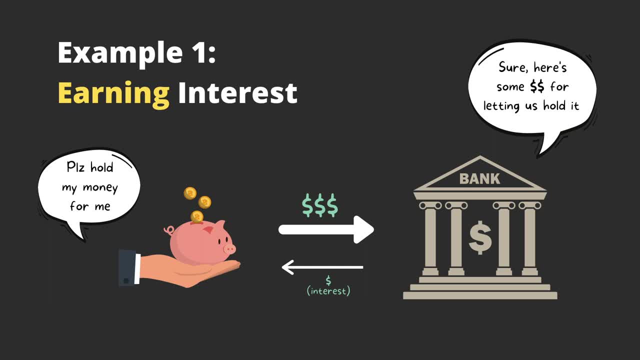 keeping your money with them. They're basically saying thanks for choosing us and letting us handle your money. here's a little bit of extra cash for banking with us. This money that you get from interest, you get to keep, which is basically free money, But on the other hand, if you borrow, 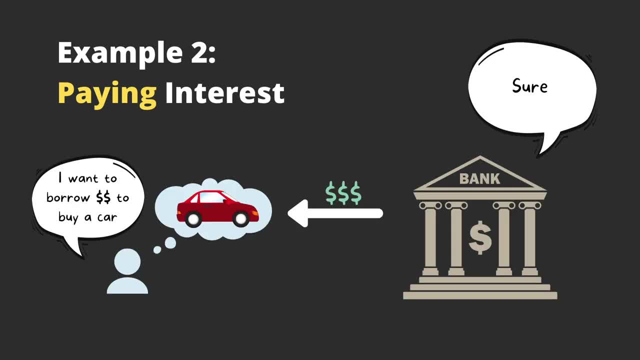 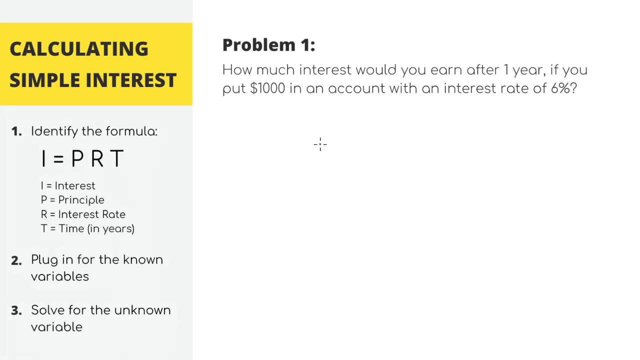 money from the bank. for example, if you took out a loan when buying a car, they will charge you an interest, or in other words, a fee for borrowing their money. This is money that you have to pay on top of what you originally borrowed. All right, let's look at some word problems. 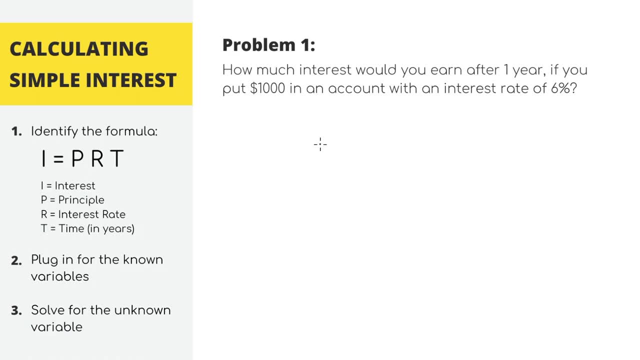 How much interest do you earn after one year if you put $1,000 in the bank with an interest rate of 6%? There is actually a formula you can use to calculate interest. It's: I equals P-R-T, where I is the amount of interest or money that you'll earn. 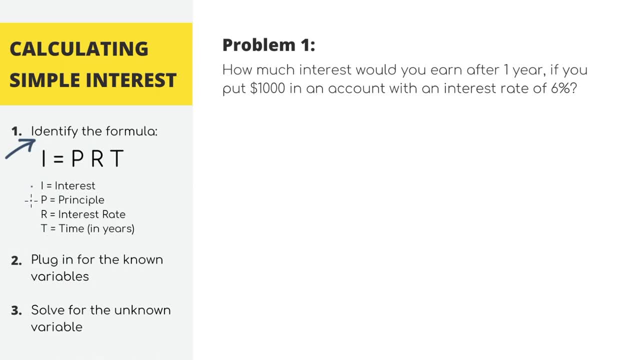 P is the principal, which is the amount of money that you first put in, R is the interest rate and T is the amount of time that you first put in, And that's the amount of time your money is in that account in years. 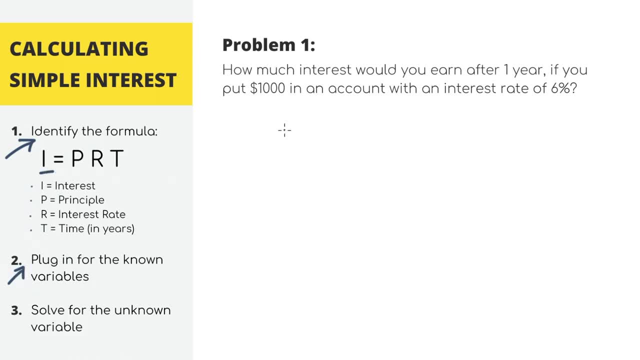 So for a problem we are trying to find, I, which is the interest we'll earn. P is the principal, or in other words the amount of money we first put in, which is $1,000.. R is the interest rate, which is 6%. 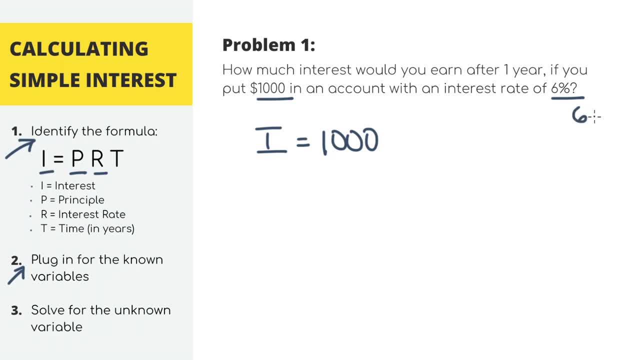 Now this is super important. Make sure you always convert the percent to a decimal. move the decimal to the left two spots. So 6% as a decimal is 0.06.. And T is the time the money is in the account, which is one year. 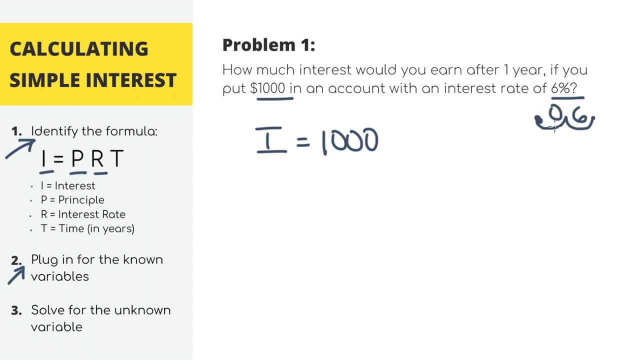 decimal to the left two spots. So 6% as a decimal is 0.06.. And t is the time the money is in the account, which is one year. Multiplying it all together, we'll get 60.. This means that if we put $1,000 into an account at this bank and wait for one, 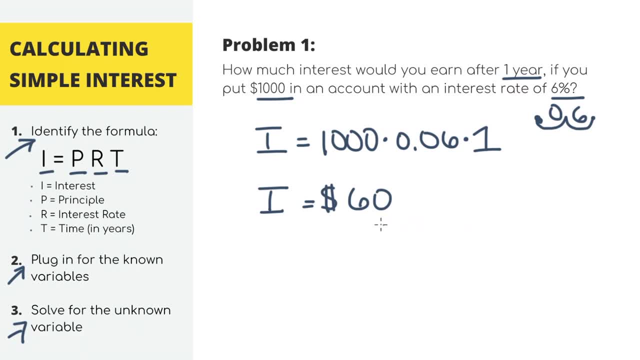 year we'll get an interest of $60, which is our final answer. Unfortunately, all these math problems you usually see are lying to you, because in the real world the interest rate is a lot lower. The very highest interest rates you can usually find is around 0.5%. So if we were to calculate our 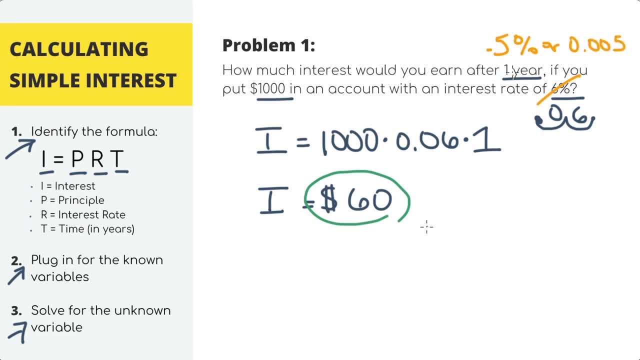 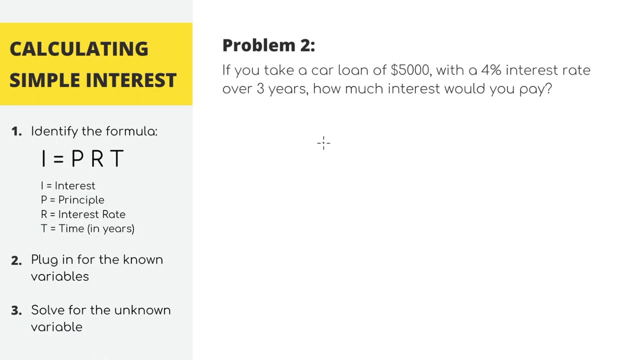 interest earned using the more realistic rate of 0.5%, we'll actually get that our interest is only $5 for the entire year, So it's not that easy getting free money. Fortunately, and also unfortunately, depending on how you look at it. this 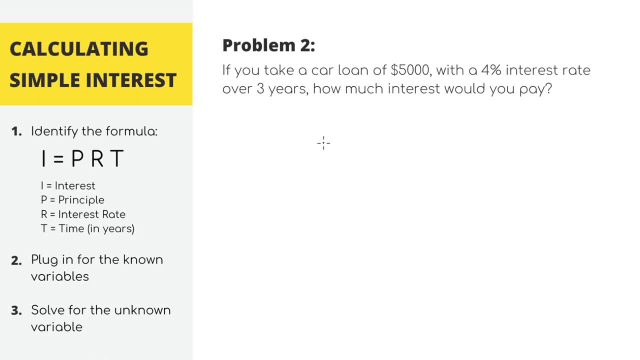 same formula works when you borrow money too. Let's say, you really want to buy a car for $5,000, but you don't have the money right now. so you take out a loan. By taking out a loan, you are borrowing money from the bank. So the bank says: 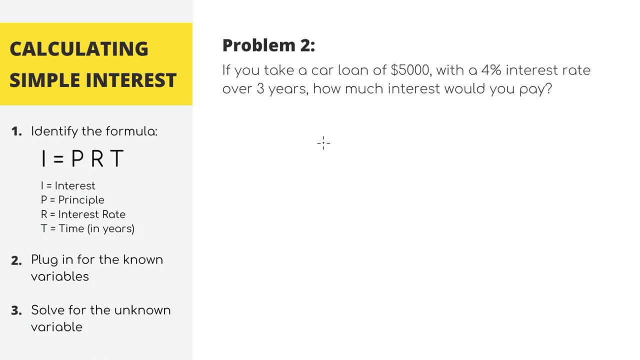 okay, you can borrow my money, but you have to pay me a $4,000. interest rate and take your time, pay me back over the span of three years. 4% doesn't sound like that much and you have some time to pay it back, but let's. 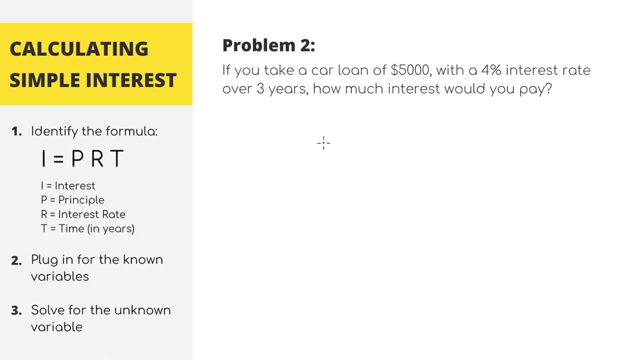 actually calculate how much extra you have to pay an interest over these three years. We're going to use the same equation: I equals PRT. We're still trying to find I, which is the interest we're going to be paying. P is the principal, which is the amount of money we're borrowing. 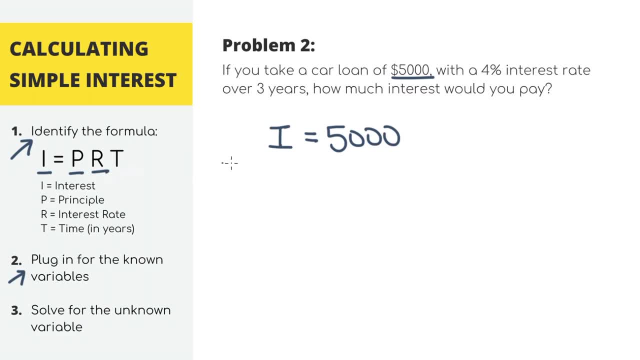 borrowing, which is 5,000.. R is the rate at .04.. And T is time, which is 3 years. When we multiply it all out, our interest is $600,, which is our final answer to this problem. 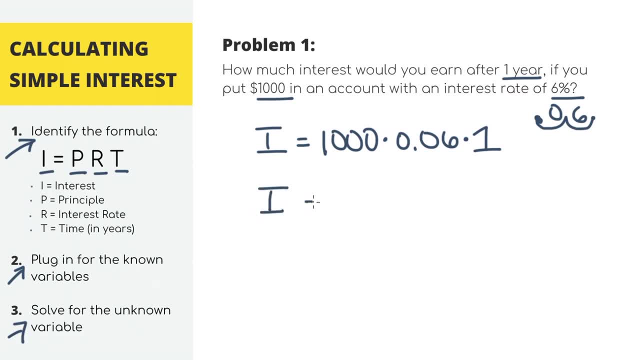 Multiplying it all together, we'll get 60. This means that if we put $1,000 into an account at this bank and wait for one year, we'll get an interest of $60, which is our final answer. Unfortunately, all these math problems you usually see are lying to you because 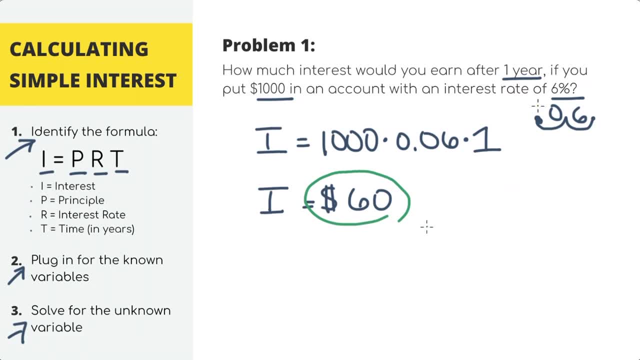 in the real world, the interest rate is a lot lower. The very highest interest rates you can usually find is around 0.5%. So if we were to calculate our interest earned using the more realistic rate of 0.5%, we'll actually. 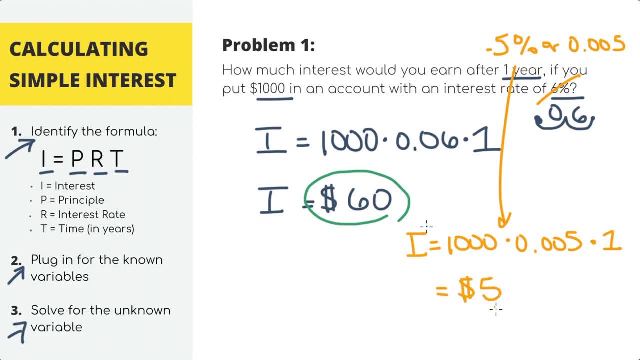 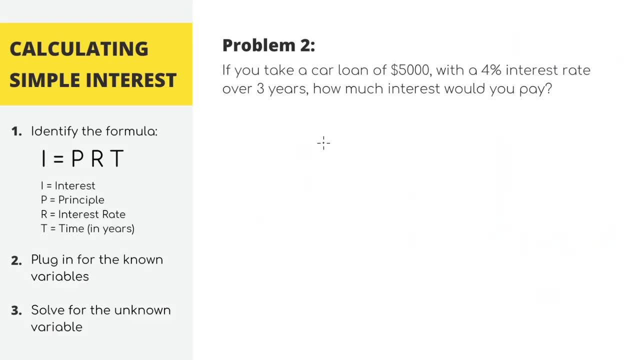 get that. our interest is only $5 for the entire year, So it's not that easy getting free money. Fortunately- and also unfortunately, depending on how you look at it- this same formula works when you borrow money too. Let's say, you really want to buy a. 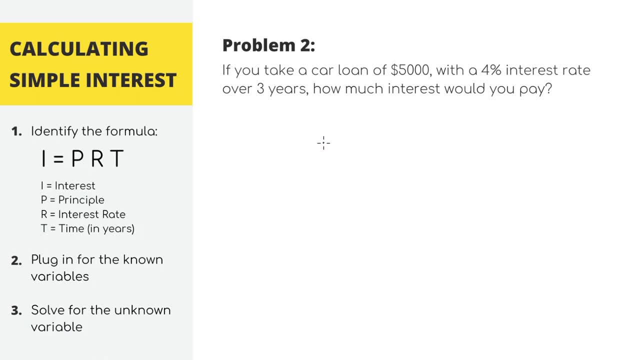 car for $5,000, but you don't have the money right now. so you take out a loan. By taking out a loan, you are borrowing money from the bank. So the bank says, okay, you can borrow my money, but you have to pay me a $4,000. 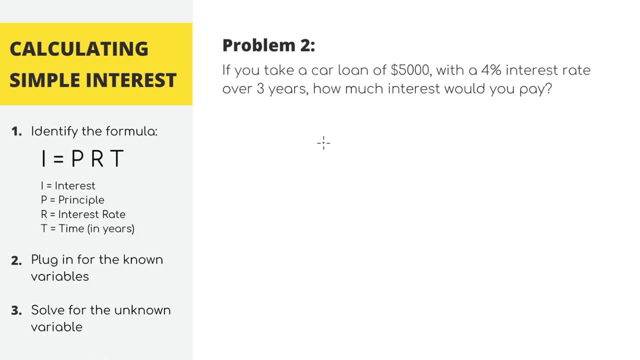 interest rates and take your time, pay me back over the span of three years. Four percent doesn't sound like that much and you have some time to pay it back. but let's actually calculate how much extra you have to pay an interest over these three years. 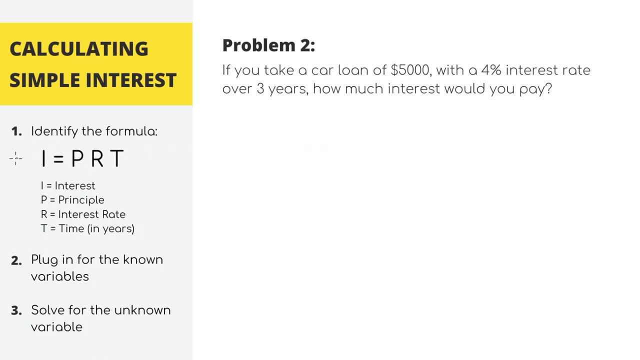 We're going to use the same equation: I equals PRT. We're still trying to find I, which is the interest we're going to be paying. P is the principle, which is the amount of money we're borrowing, borrowing which is 5,000.. R is the rate at .04.. And T is time, which is 3 years, When. 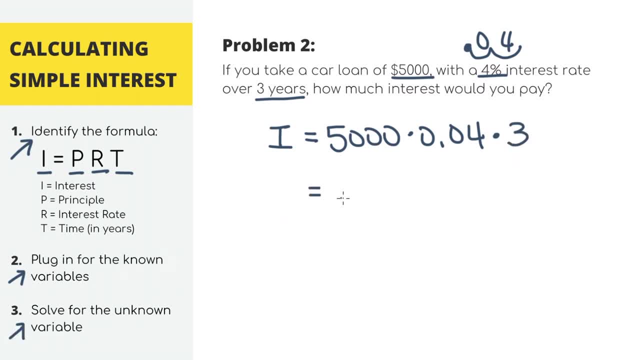 we multiply it all out. our interest is $600,, which is our final answer to this problem, And this means that you are paying $600 more to be able to borrow the money. So over the span of 3 years, you'll be paying a total of $5,600 instead of just $5,000 if you didn't. 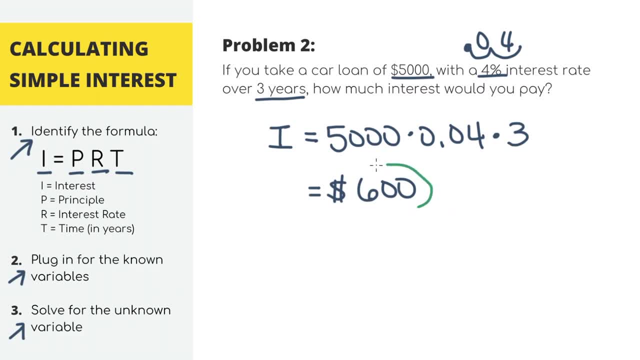 And this means that you are paying $600 more to be able to borrow the money. So over the span of 3 years, you'll be paying a total of $5,600 instead of just $5,000 if you didn't have to take out the loan. 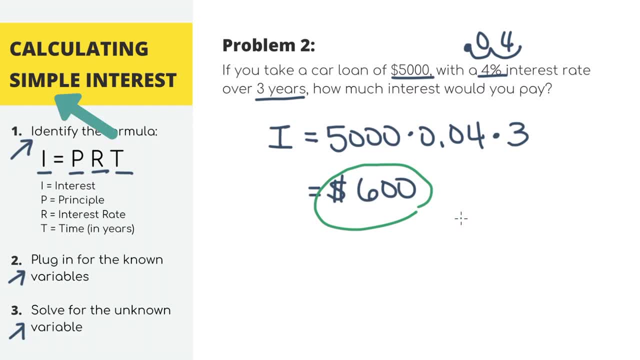 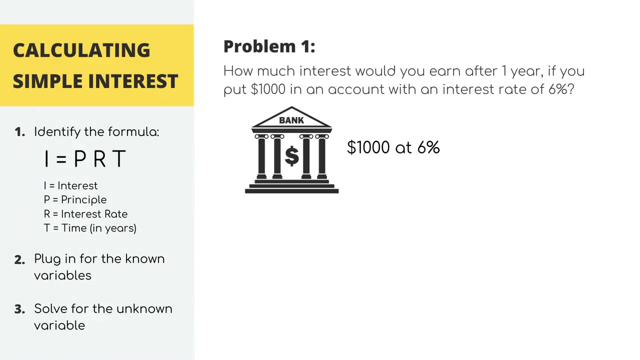 Now, what we just learned is called simple interest. There's also something called compound interest, where you're earning interest on top of your interest. So, for example, if we go back to the scenario where we put $1,000 in the bank with 6% interest, let's say the. 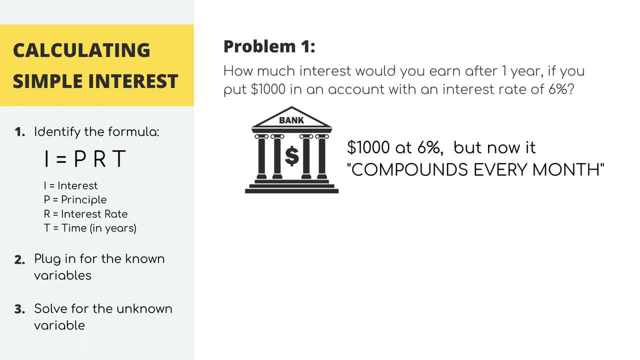 bank uses compound interest and it compounds every month. That means if we put the money in in January, by the end of the month we're going to have $1,005.. So this is how it was with simple interest. also, In the next month we're still getting 6% interest, but now it's. 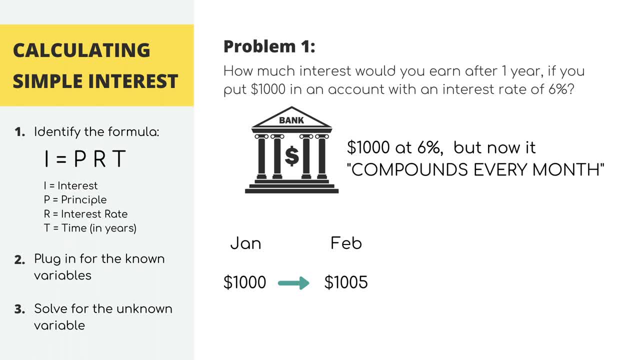 6% interest on $1,000.. So by the end of February we'll have $1,010.02 in the account. This additional 2.5 cents is because of the compounding. If we keep compounding every month by the end of the 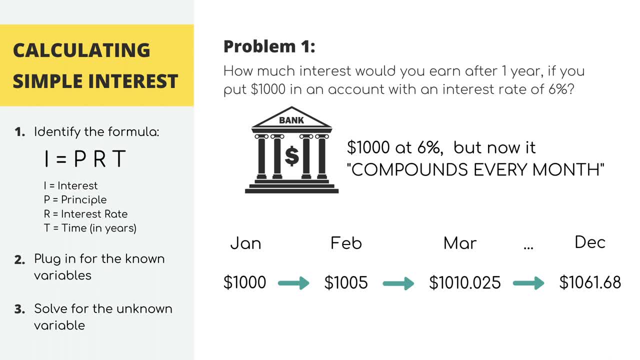 year in December we're going to have $1,061.68 instead of just the $1,060 we got from simple interest, This amount seems small, but when we're talking about much bigger numbers like $10,000, $100,000,. 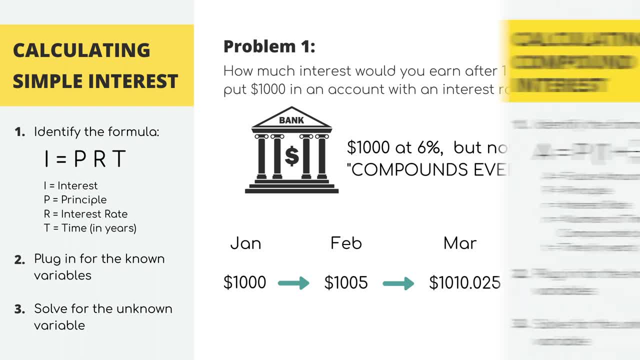 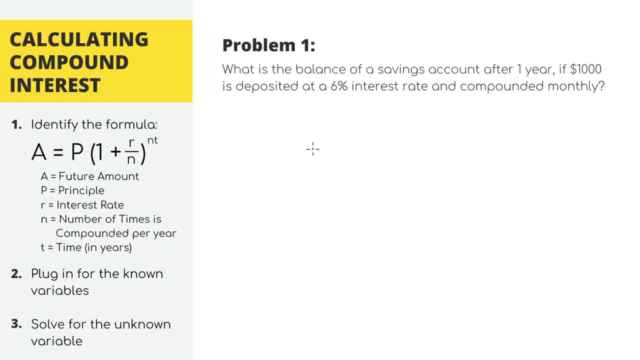 or even $1,000,000, it definitely adds up. If we were to put what we just calculated into a normal problem you might see in class it would look something like: how much money would there be in a savings account after one year if $1,000 is deposited at a 6% interest rate, compounded monthly For compound interest? 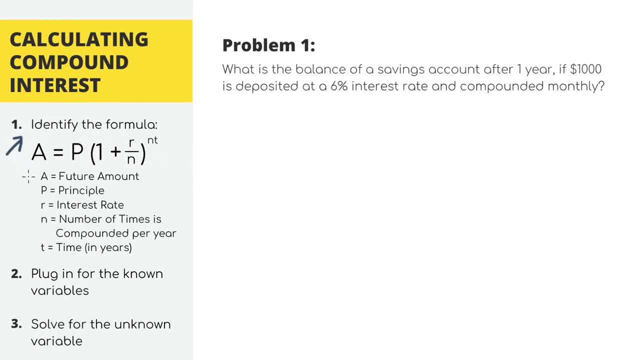 we have a new formula. now The future amount or the total amount of money we're going to have in the account P is still the principal, which is the amount of money we're first putting in. R is still the interest rate in decimal form, but now we have a variable called n, where n is the 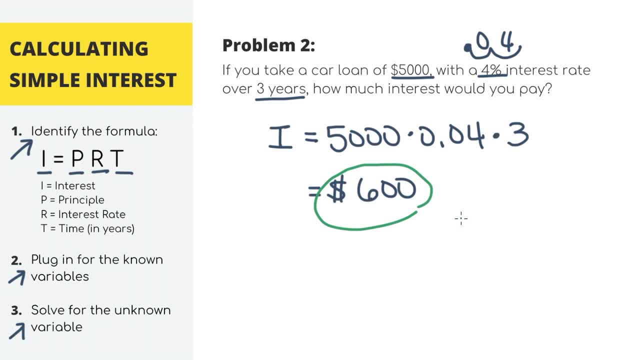 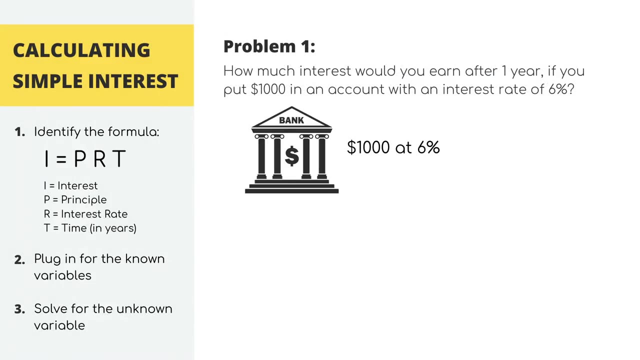 have to take out the loan. Now, what we just learned is called simple interest. There's also something called compound interest, where you're earning interest on top of your interest. So, for example, if we go back to the scenario where we put $1,000 in the bank with 6% interest, let's say the 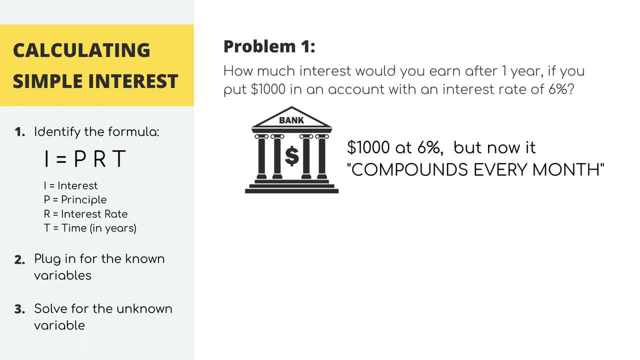 bank uses compound interest and it compounds every month. That means if we put the money in in January, by the end of the month we're going to have $1,005.. So this is how it was with simple interest. also, In the next month we're still getting 6% interest, but now it's. 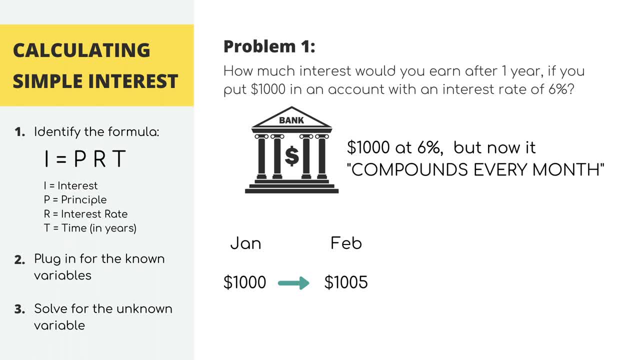 6% interest on $1,000.. So by the end of February we'll have $1,010.02 in the account. This additional 2.5 cents is because of the compounding. If we keep compounding every month by the end of the 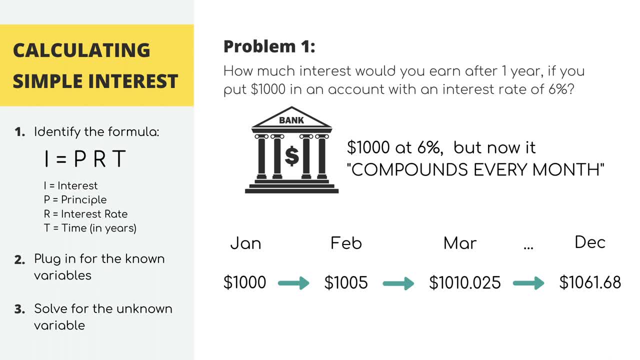 year in December we're going to have $1,061.68 instead of just the $1,060 we got from simple interest, This amount seems small, but when we're talking about much bigger numbers like $10,000, $100,000,. 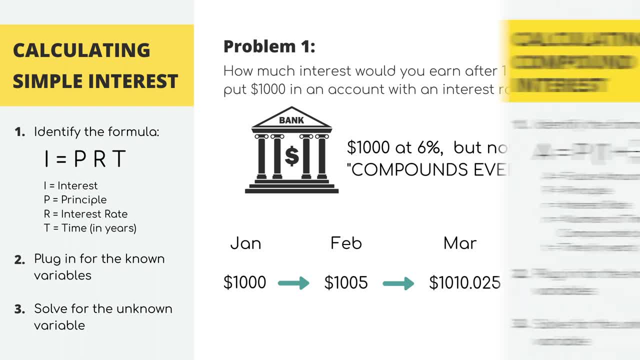 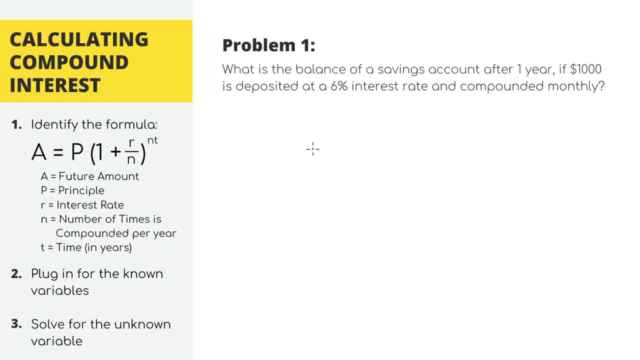 or even $1,000,000, it definitely adds up. If we were to put what we just calculated into a normal problem you might see in class it would look something like: how much money would there be in a savings account after one year if $1,000 is deposited at a 6% interest rate, compounded monthly For compound interest? 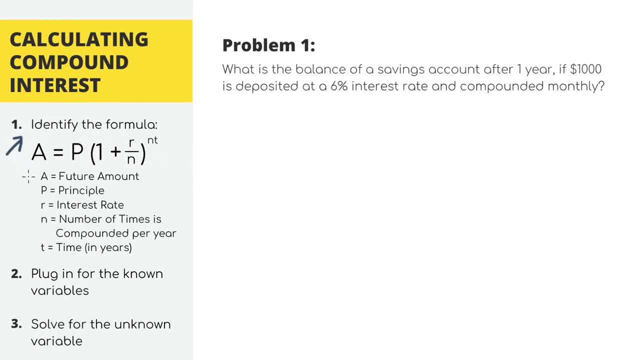 we have a new formula. now The future amount or the total amount of money we're going to have in the account P is still the principal, which is the amount of money we're first putting in. R is still the interest rate in decimal form, but now we have a variable called n, where n is the 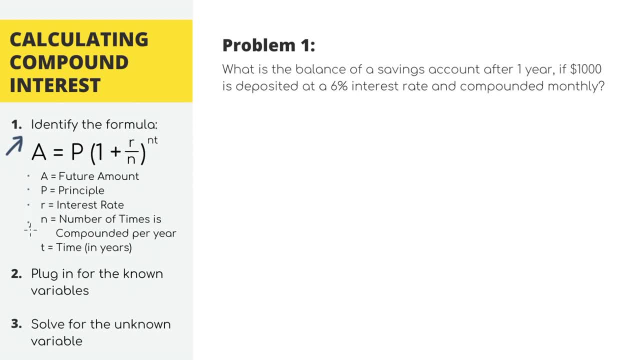 number of times. it's compounded per year and t is still time in years. And plugging in all the numbers we're solving for a P equals $1,000.. R equals .06.. N equals 12, because it's compounded monthly and there are 12 months in a year. 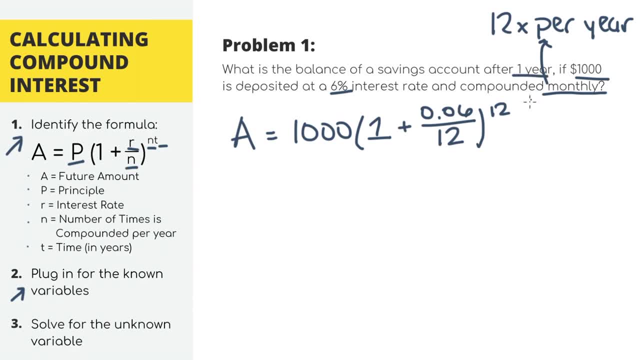 And T is the time the money is in the account. P equals $1,000.. which is 1 year. We'll get our answer $1,061.68.. That means we'll have $1,061.68 in our bank. 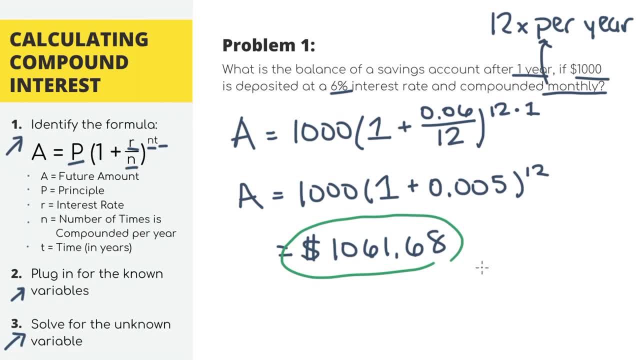 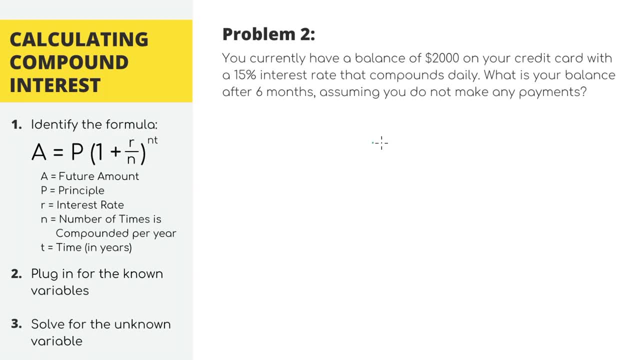 account after 1 year, which is great- more money. Now, compound interest gets pretty scary when you think about loans and when you're borrowing money, because you'll end up owing more. Credit card companies, for example, use compound interest, which means that you're paying interest on top. 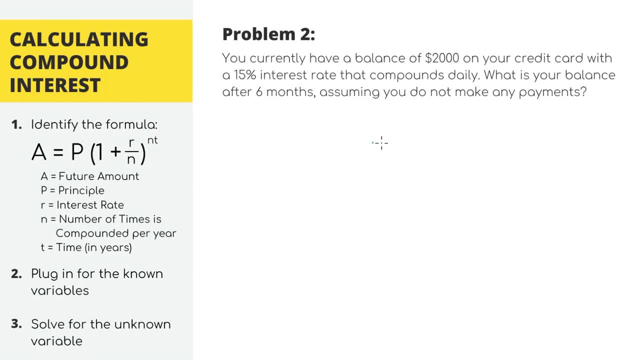 of your interest when you don't pay them back. Credit card companies are also notorious for having super high interest rates too. So let's say you charged $2,000 to your credit card, which is basically temporarily borrowing $2,000 from them. Your credit card has a 15% interest. 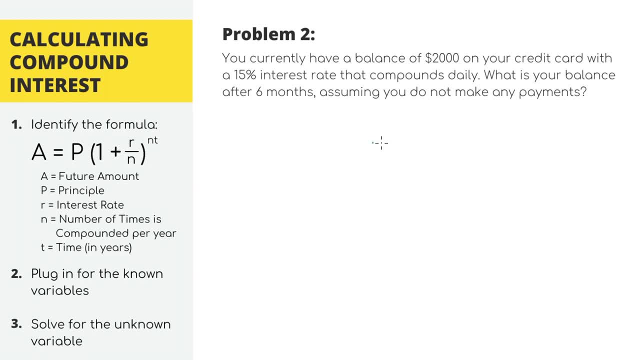 rate that compounds daily, which I could say is fairly standard in the real world, How much money would you owe in 6 months if you don't make any payments towards it? We can use our compound interest equation to get the answer. We're trying to solve for A, which is our future. 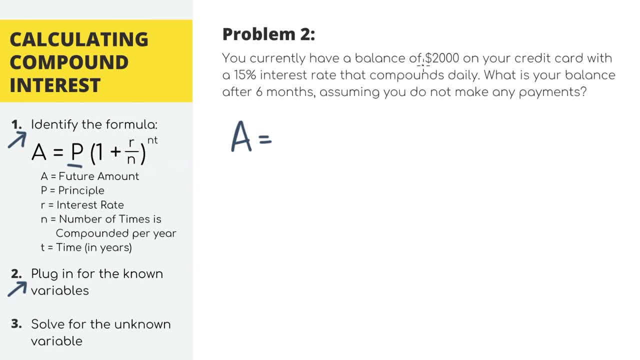 amount. P equals 2,000, because that's the initial amount we charged to the credit card. R equals 0.15.. N equals 365, because N is the number of times it compounds each year. So if it compounds daily, then it compounds 365 times per year. And T equals 0.5 years, because 6 months is one half of a year. 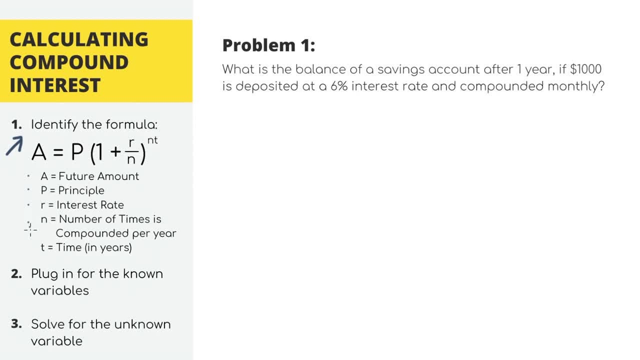 number of times. it's compounded per year and t is still time in years. And plugging in all the numbers we're solving for a P equals 1000.. R equals .06.. N equals 12. Because it's compounded monthly. 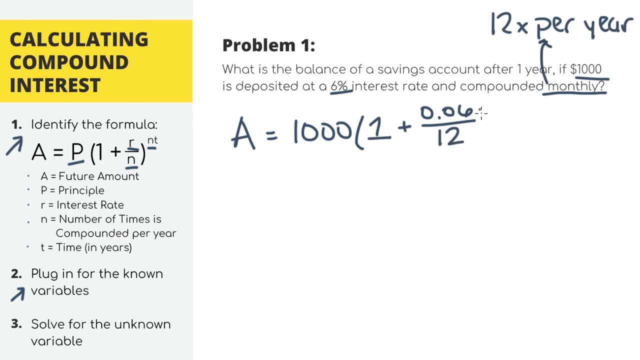 There are 12 months in a year And t is the time the money is in the account. Christmas Yes, which is 1 year. We'll get our answer $1,061.68.. That means we'll have $1,061.68 in our bank. 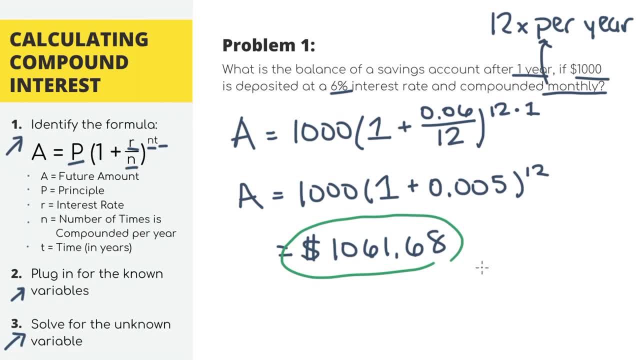 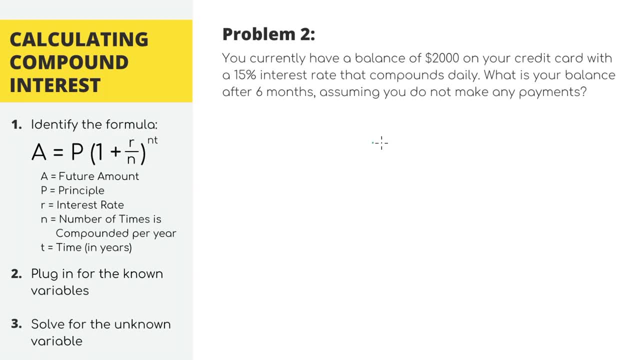 account after 1 year, which is great- more money. Now, compound interest gets pretty scary when you think about loans and when you're borrowing money, because you'll end up owing more. Credit card companies, for example, use compound interest, which means that you're paying interest on top. 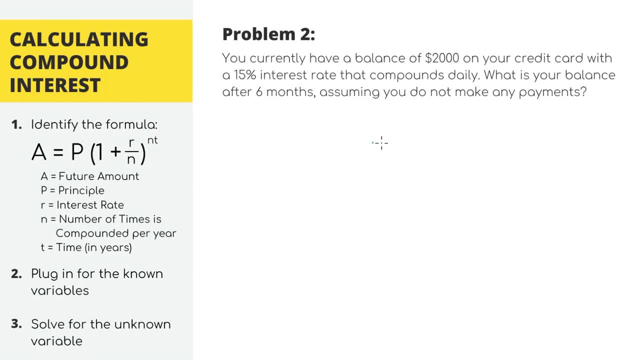 of your interest when you don't pay them back. Credit card companies are also notorious for having super high interest rates too. So let's say you charged $2,000 to your credit card, which is basically temporarily borrowing $2,000 from them. Your credit card has a 15% interest. 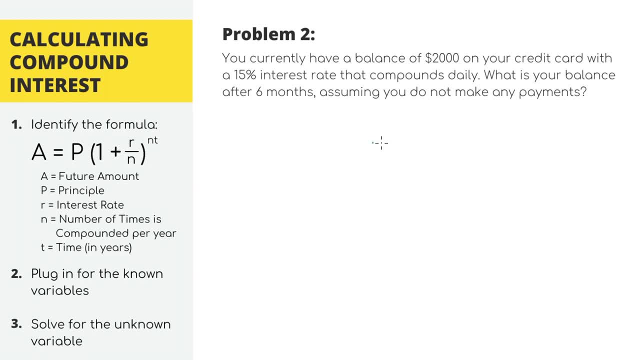 rate that compounds daily, which I could say is fairly standard in the real world, How much money would you owe in 6 months if you don't make any payments towards it? We can use our compound interest equation to get the answer. We're trying to solve for A, which is our future. 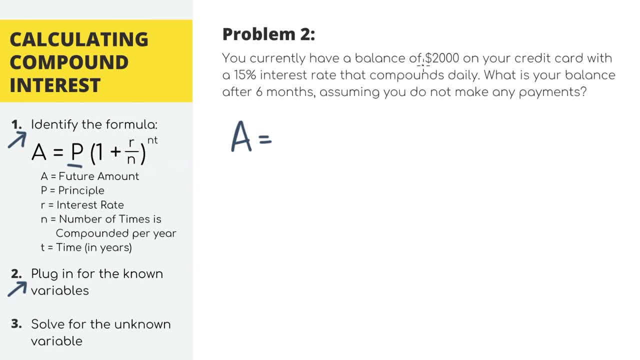 amount. P equals 2,000, because that's the initial amount we charged to the credit card. R equals 0.15.. N equals 365, because N is the number of times it compounds each year. So if it compounds daily, then it compounds 365 times per year. And T equals 0.5 years, because 6 months is one half of a year.